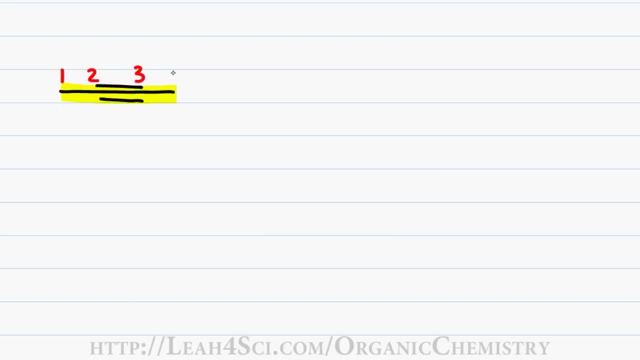 of the molecule. I can start numbering from the right or the left and I have a total of four carbons, giving me a first name of bute, Because I have a triple bond in the molecule. I get a last name of Yne or Ine. I place number two in front of the Ine. this way I can then. 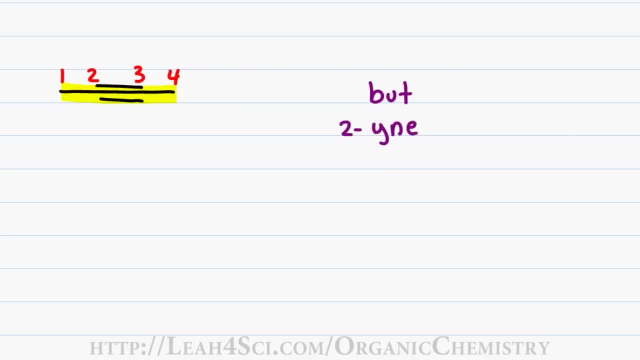 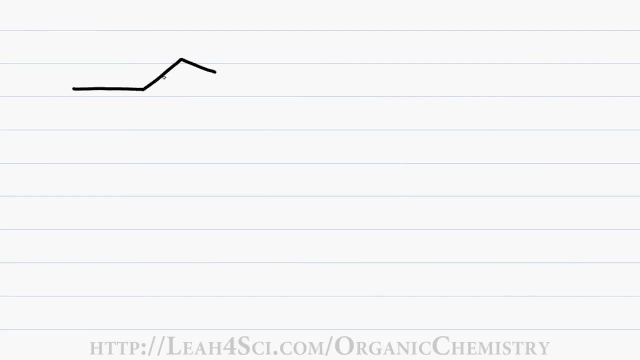 specify where the triple bond occurs on the molecule and this gives me a final name of 2-butyne. Let's try another example. For this example, recognize that we have a terminal alkyne because the triple bond is at the end of the molecule. I start by highlighting the 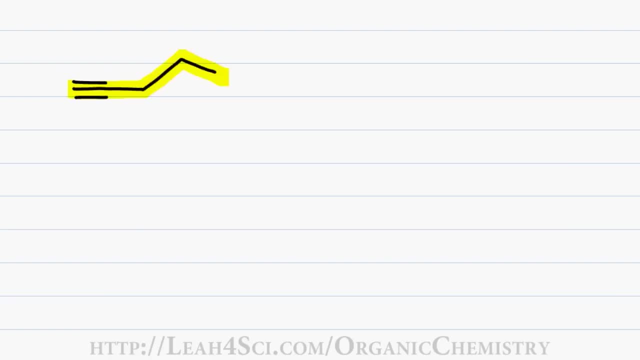 parent chain. When the alkyne is your highest priority, you start numbering from the side. that will give it the lowest number. I start numbering from the left and get a total of 5. for a first name of Pent. Since the triple bond occurs on number 1, I have 1-Ine. for a final name of 1-Pentine. 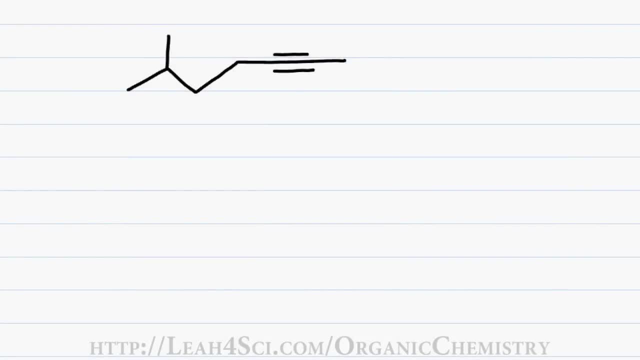 For this example, I have a substituted alkyne and once again I start by highlighting my parent chain. I have the option of numbering from the left, where I had a methyl group at Carbon-2, or numbering from the right, where I had the alkyne at Carbon-2.. When you have 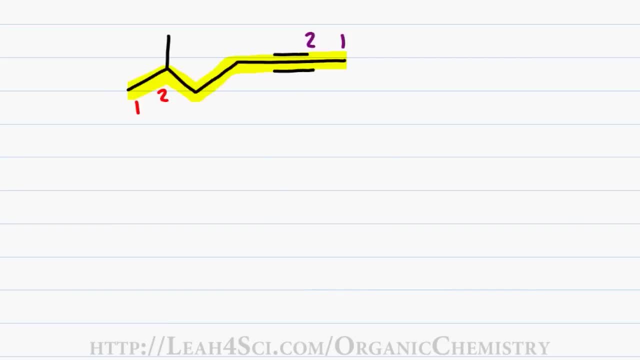 a substituent and a triple bond. you start numbering from the left. where I hit a methyl bond that both have the same number, the substituent gets highest priority and that means I have to start numbering from the left. 7 carbons in my parent chain gives me a first name of 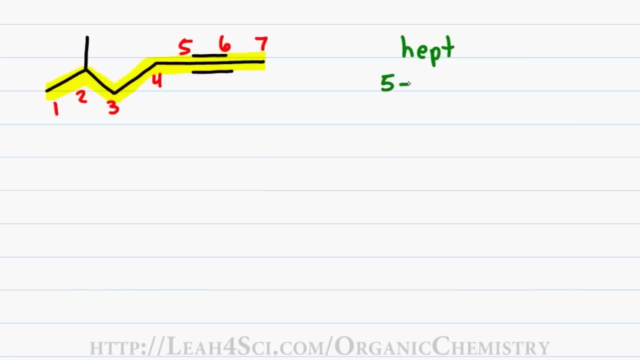 hept. Getting my triple bond at carbon 5 gives me a last name of 5-ine and my methyl group substituent on carbon 2 gives me 2-methyl. Putting the name together, I have 2-methyl-5-heptine. 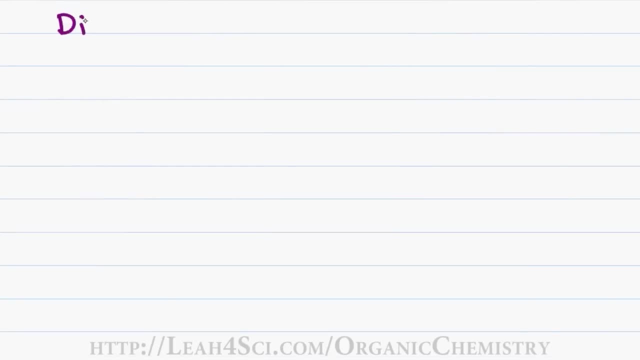 A di-ine is not as scary as it sounds. it simply means that you have two carbon to carbon triple bonds on the same molecule. We'll use this molecule as an example and once again, we start by highlighting the parent chain. In this case, I have a terminal alkyne on. 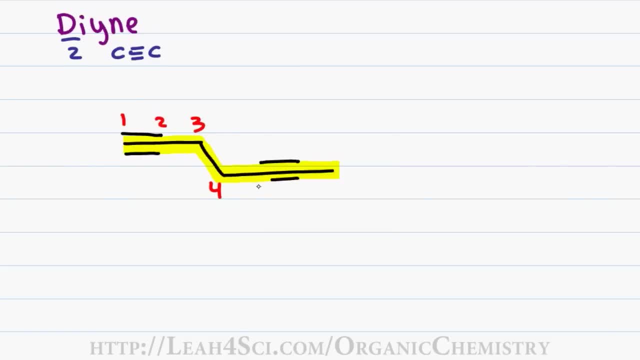 the left, and so we start numbering from the left to get a total of 7 carbons for a first name of hept. Since I have two triple bonds occurring on carbon 1 and carbon 2, I have to include both numbers, giving me 1,5.. I start with the last name of di-ine to show that.